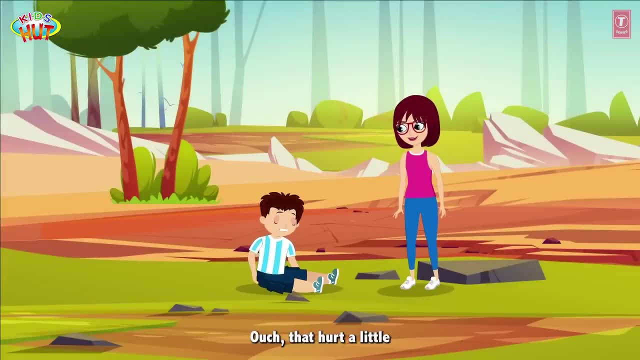 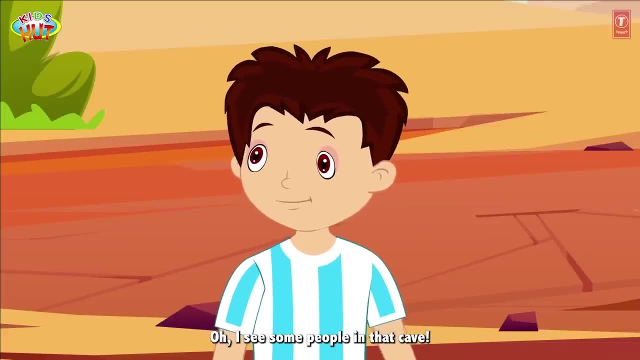 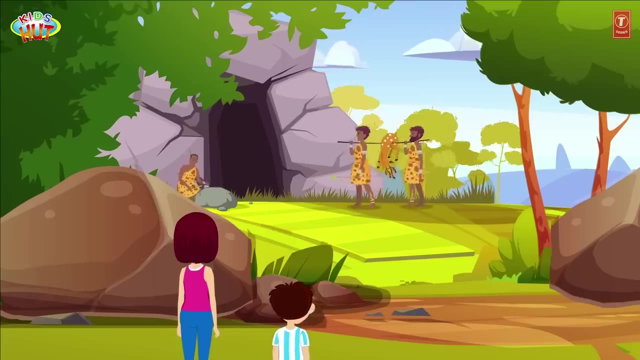 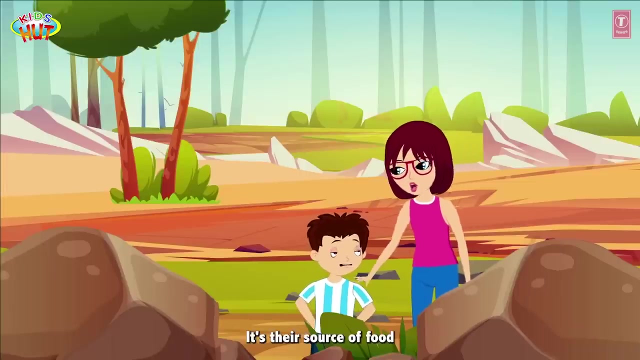 Ouch, That hurt a little. Oh, Tofu, Let's look around. Oh, I see some people in that cave. Tia, why did they kill the poor deer? It's their source of food. They hunted animals, cooked the meat. 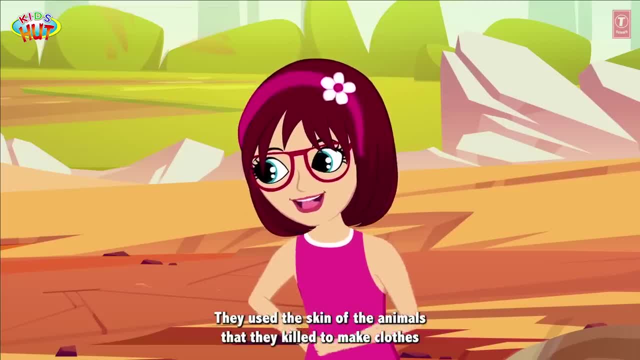 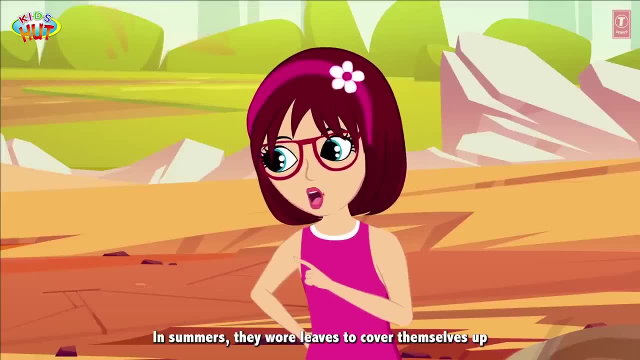 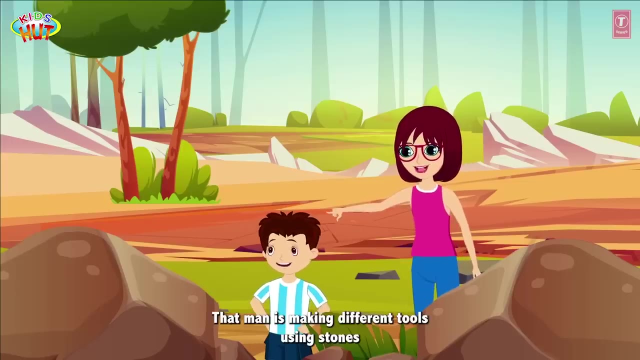 and filled their stomachs. They used the skin of the animals that they killed to make clothes in order to protect themselves from the weather. In summers, they wore leaves to cover themselves up. Oh, Look there, That man is making different tools using stones. 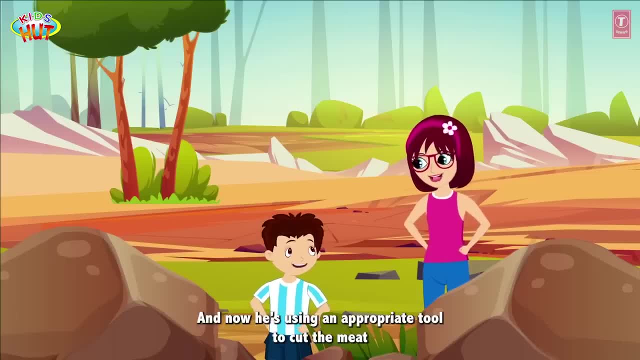 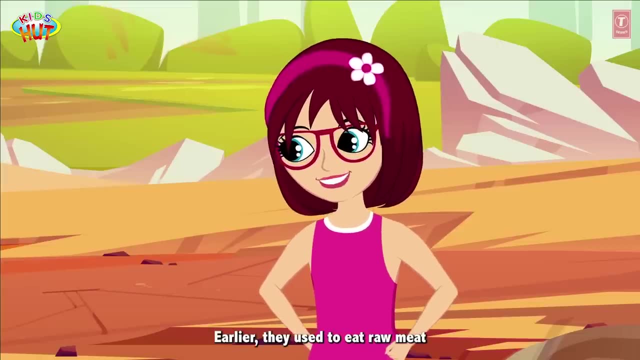 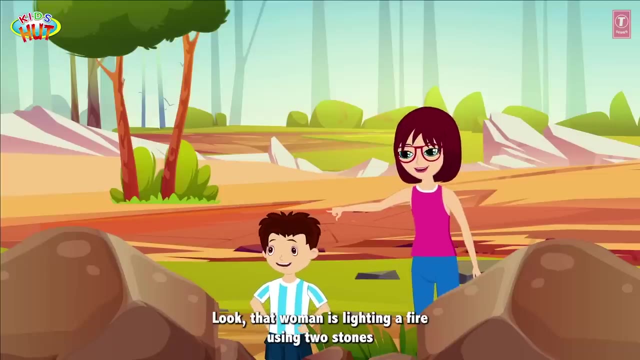 And now he is using an appropriate tool to cut the meat. Will they eat it raw? Well, earlier they used to eat raw meat, But then they discovered fire to cook and keep themselves warm. Look that woman is lighting a fire using two stones. 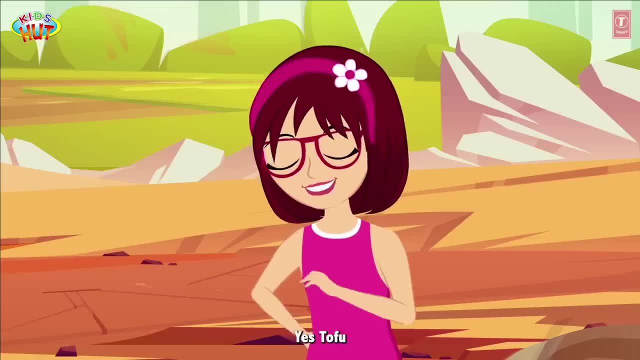 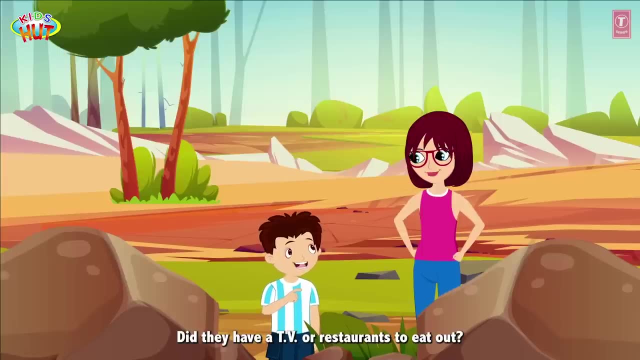 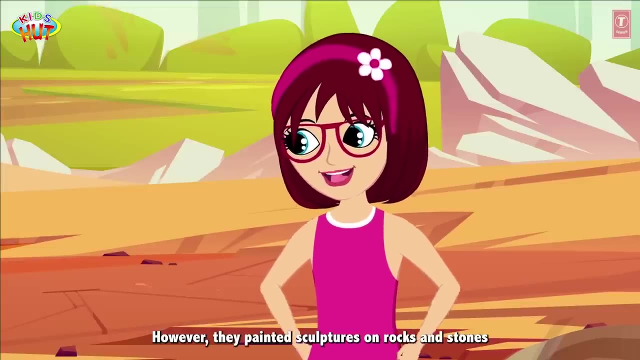 Wow, That's amazing. Yes, Tofu Tia. what did they do in their free time? Did they have a TV or restaurants to eat out? Oh, no dear, They had no such entertainments. However, they painted sculptures on rocks and stones. 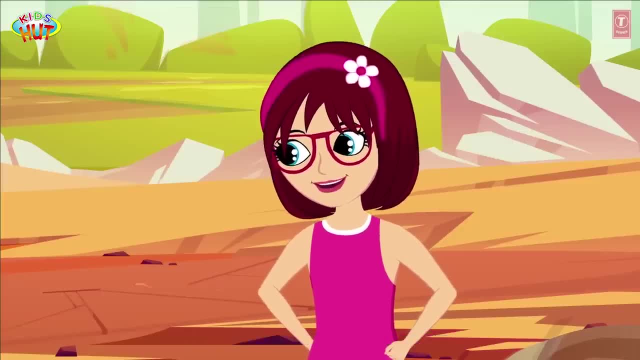 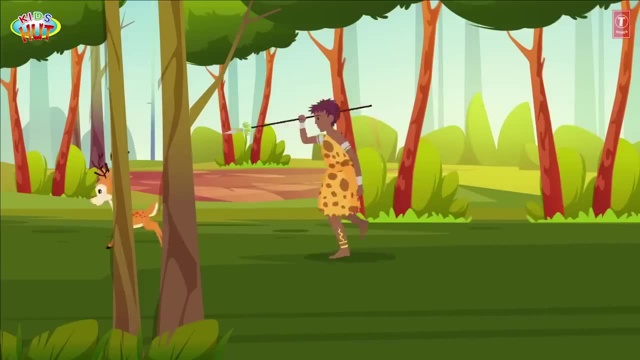 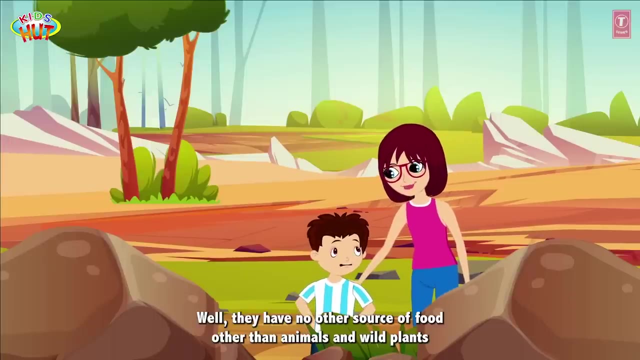 Later they even started making clay pottery. Wow, Tia, Hey, look there They are trying to hunt a deer, Poor animals. I feel so sad for them. Well, they had no other source of food other than animals and wild plants. 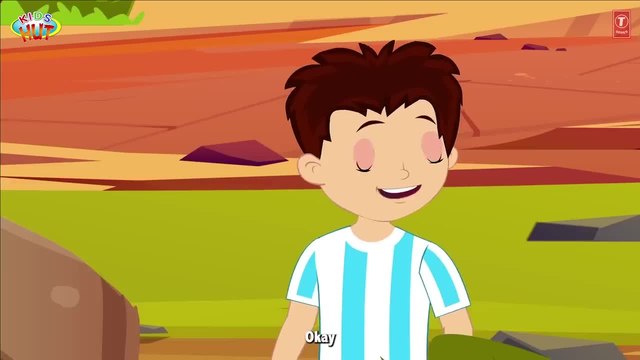 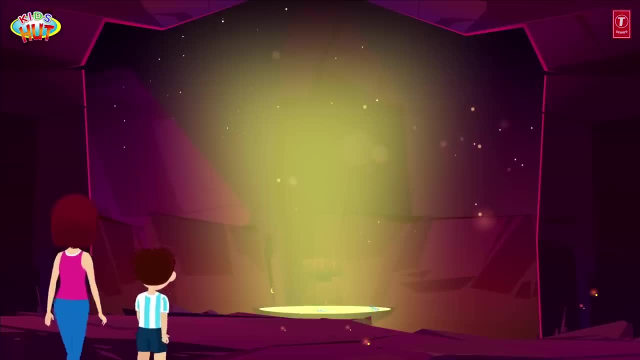 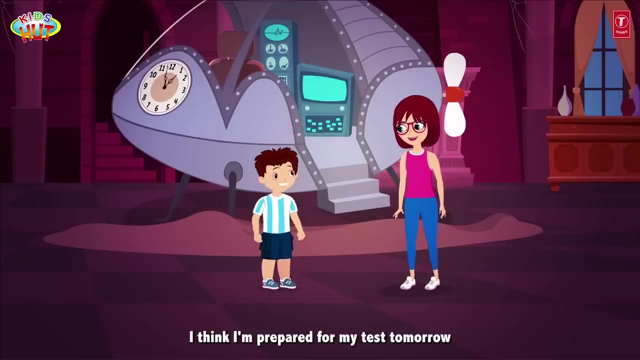 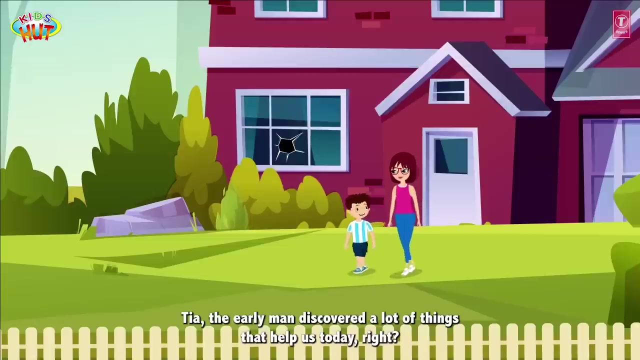 Shall we go home now, Tofu? Okay, Let's go, Tia, I think I am prepared for my test tomorrow. That's great, Tofu. Tia the early man discovered a lot of things that help us today, right. 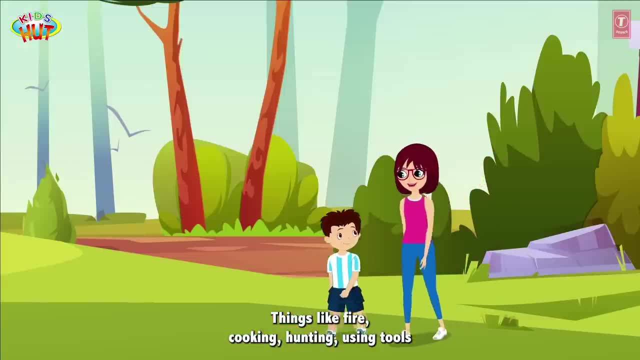 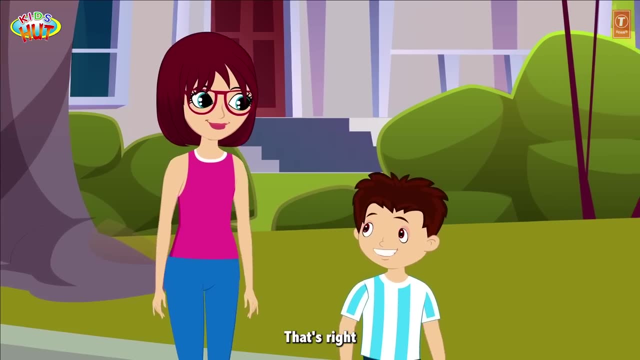 Yes, Tofu. Things like fire, cooking, hunting using tools, wearing clothes were all discovered by the early man. That's right. I think I'll get good grades in the test now. I am sure you will. All the best. Thanks Tia.